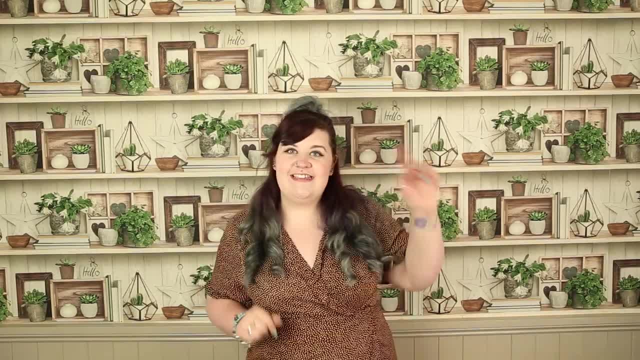 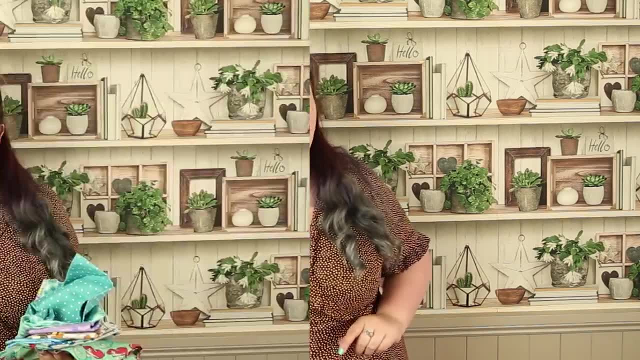 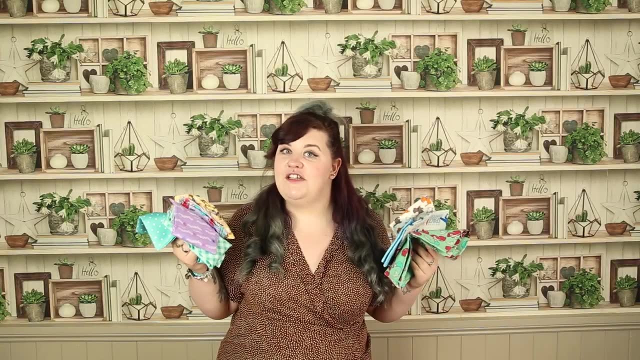 Hey, creatives, Welcome to my channel. This is Sammy Says Create and this is a channel where I do all sorts of DIY and creative projects and I bring you along for the ride. So welcome to my mini-series. This is 5 Minute Fat Quarters and this is the series where I show you some fun and fabulous fat quarter makes in 5 minutes or under. 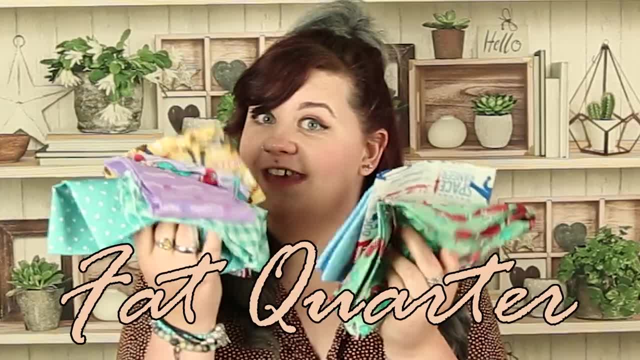 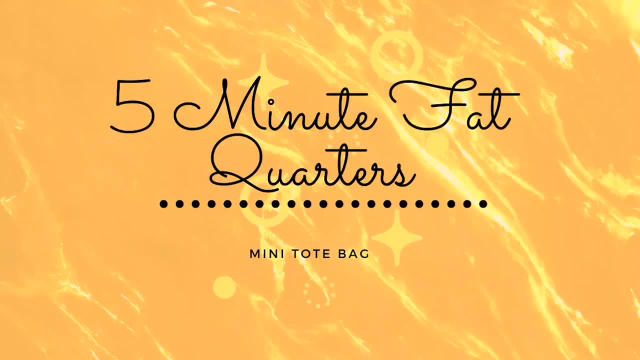 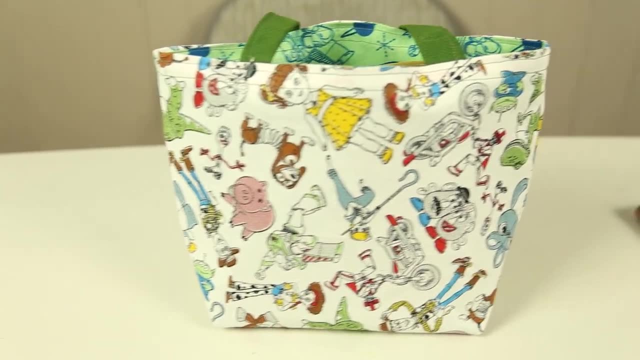 No frills, no fluff, just fat quarter. So, without further ado, let's get on with today's fat quarter make. So in today's video, I'm going to show you how to make this super, super cute mini bag. I've got loads of Disney fat quarters, so that is what I'm going to be using myself for this make. 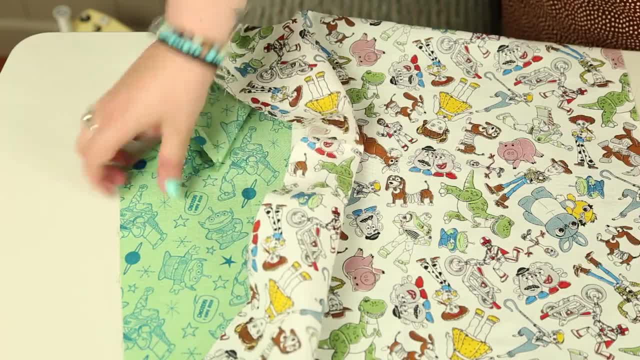 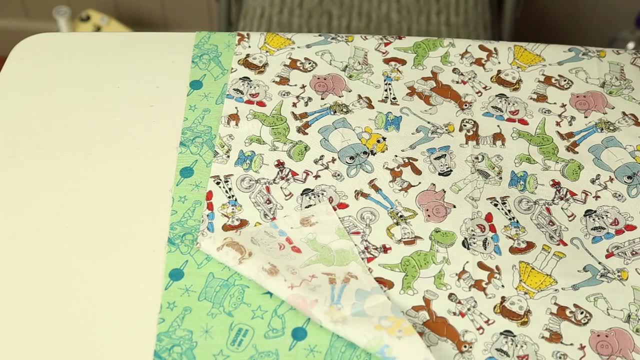 So you will need one full fat quarter in total to make this bag. I have chosen to have a different fat quarter for the lining. therefore, I'm going to use two fat quarters and cut them in half. You will also need a little bit of fat quarter to make this bag. 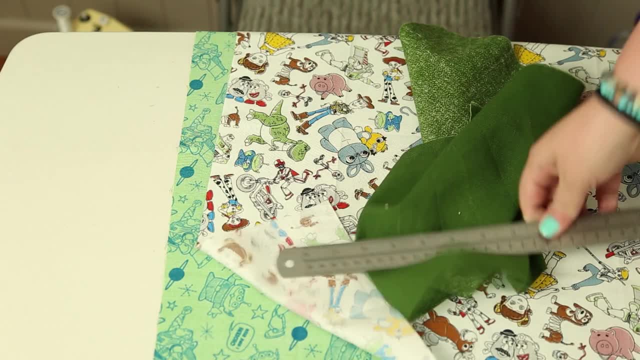 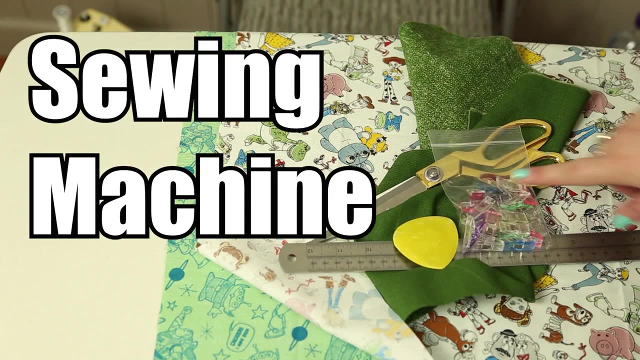 And a little bit of scrap fabric for the handle as well. In addition to this, you will need a ruler, some chalk, some fabric scissors, some clips or pins, and you will need a sewing machine. First, you need to measure your fat quarter and cut it in half, or both your fat quarters if you are using two. 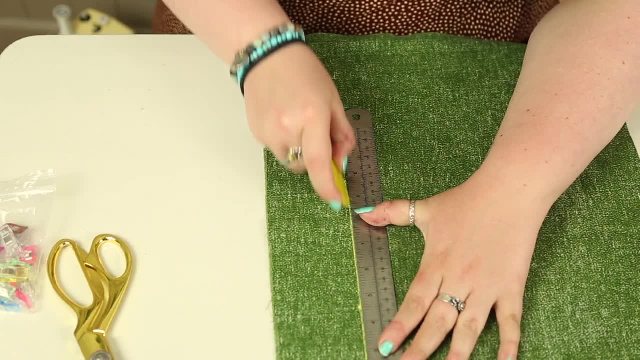 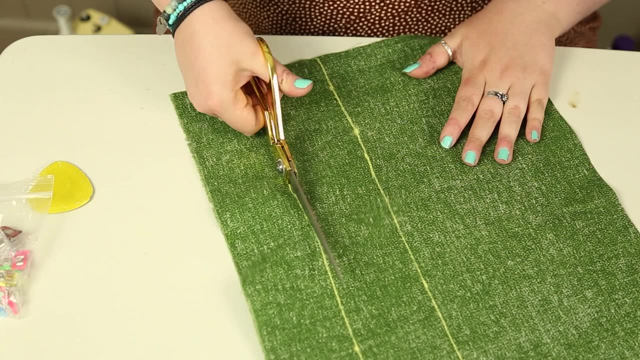 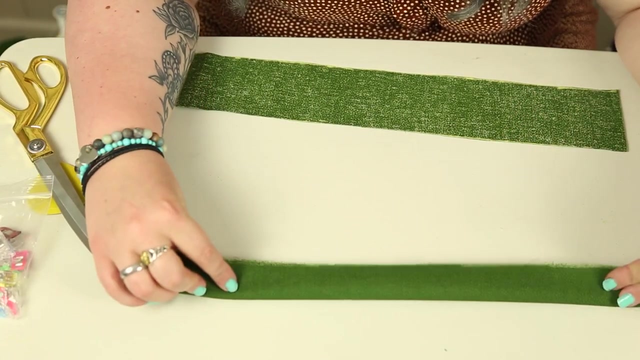 Then you need to measure and cut out the handle. So I did mine 16 inches long by 3 inches wide, but you can alter this if you feel like you want it bigger or smaller, And you will need two of these cutting out. So to carry on making our handles, you will need to fold the material in half, just to crease it. 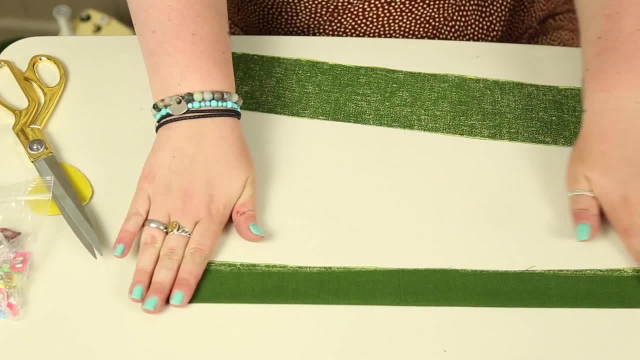 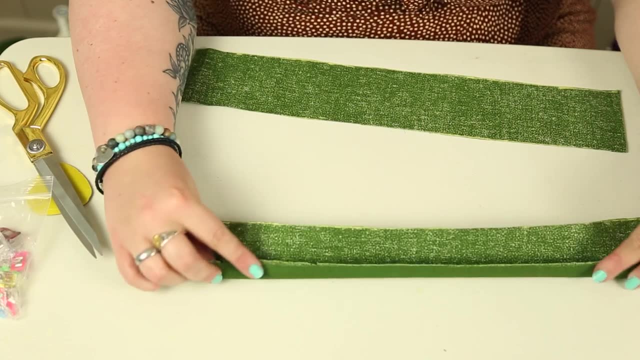 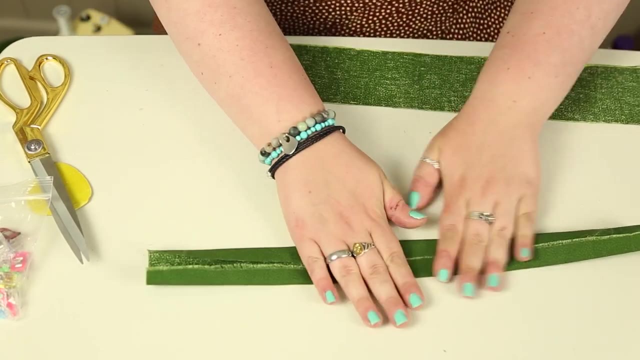 You can iron it here if you find it easier and it stays a little bit better. This material was quite good at staying in place. You're then going to open it up and you're going to fold them in half again And then just fold that whole thing. 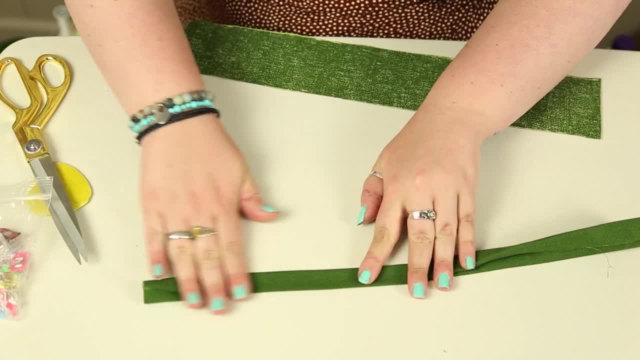 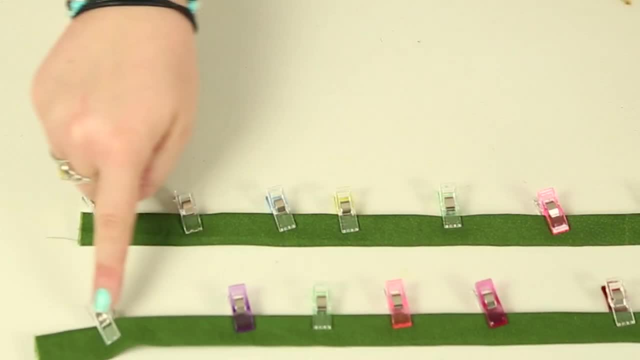 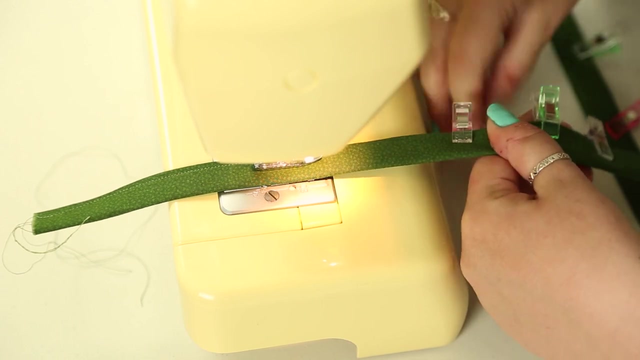 in half again. if that makes sense, then clip or pin this just to keep it nice and secure, and we're gonna do one long straight stitch across the side where the two sides are open and that will just secure it into place. you're then going to take the fat quarter that you want to be on the outside of the back. 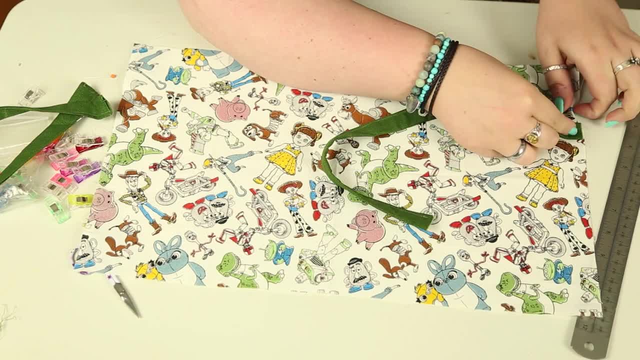 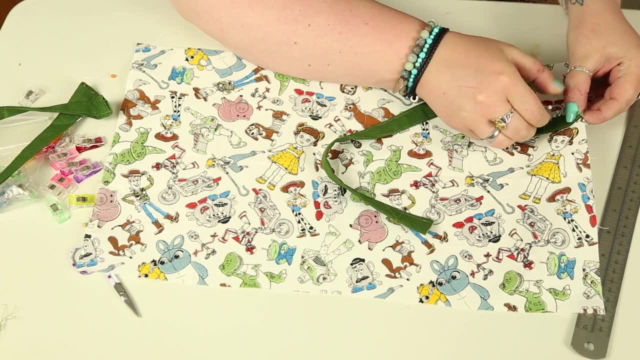 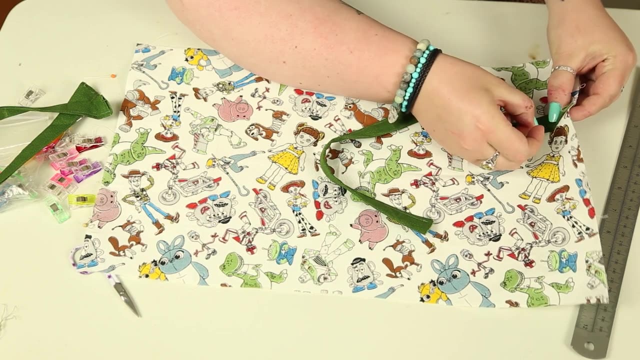 and that's gonna face upwards. then measure and pin equally the ends of the handle just to the top of the bag. make sure the pin is slightly further down so it makes sure it's not right at the top of the material. as we are going to stitch over these handles. the handles need to be facing towards the middle of. 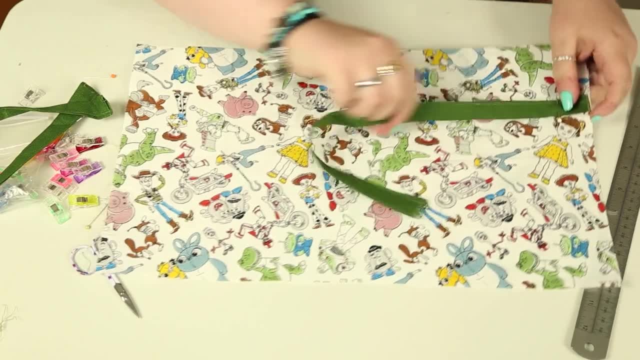 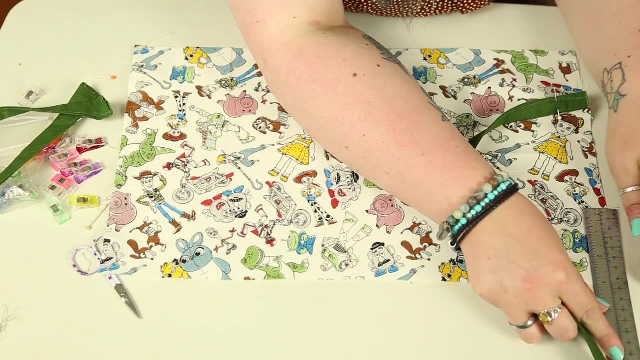 the material. and don't forget that if you've got a pattern on your material, just keep an eye on which way the pattern needs to go. if it does need to go a certain way, the middle of this material is going to be the bottom of the bag. we have our handles all pinned equally and now we need to use the other. 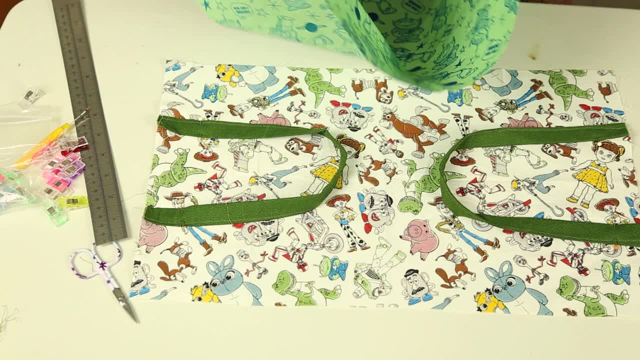 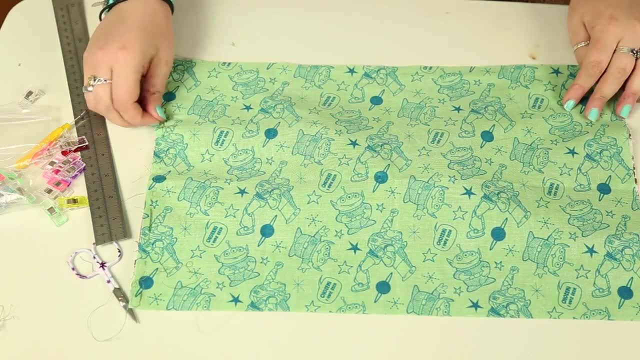 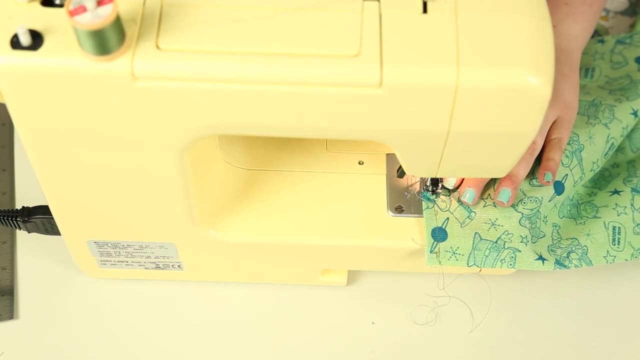 half of the material and place it on top, so it should look like this again the pattern is facing upwards- and just match this as neatly as you can. again, clip or pin just to make it nice and secure. and then we're going to do two lots of straight stitches from top to bottom on these shorter edges. then 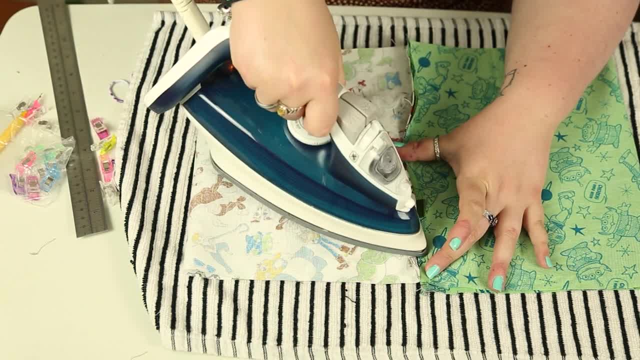 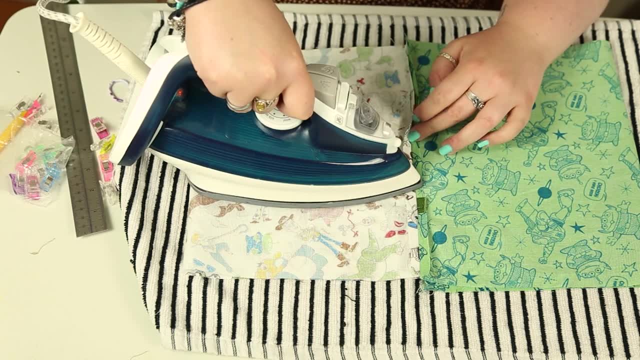 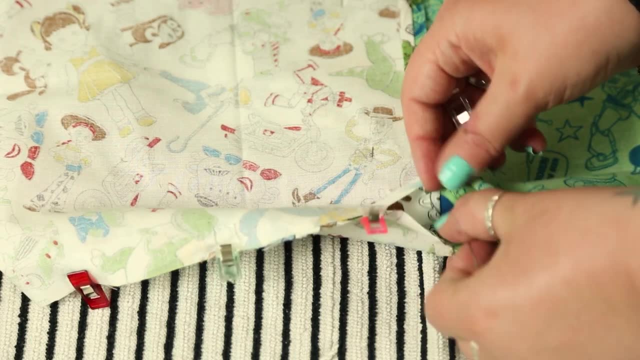 open up your material and bring those two seams that you've just stitched into the middle- so both matching pieces of material should be on either side- and just iron down that hem flat and do this on both sides, then going to clip or pin just those two longer edges together and we're going to do two straight. 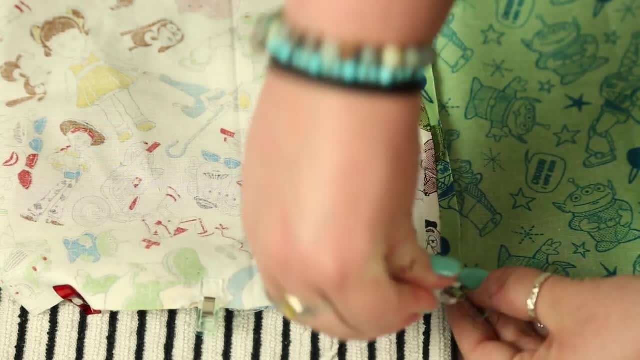 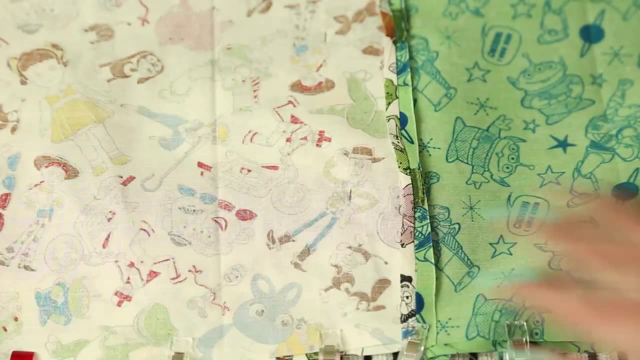 stitches across these longer edges, so make sure you leave a little gap, on whichever side you want the lining to be at the end, just so we can flip it the other way around. we are now all sewn up and I'm going to use that hole that we 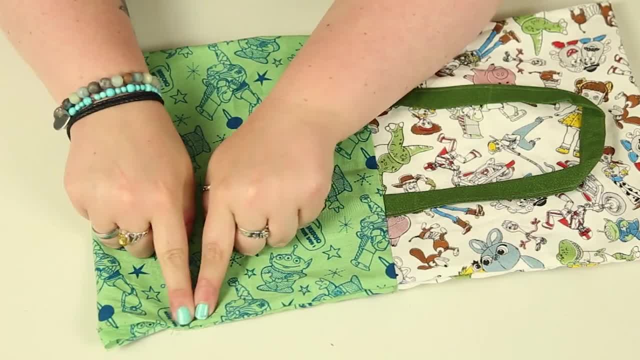 left just to flip the bag the other way around. so just do a little touch up, and then we're going to do the other side, and then we're going to do the other side, and then we're going to do the other side, and then we're going to do. 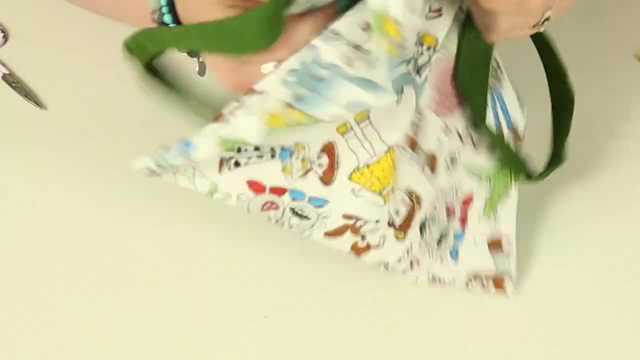 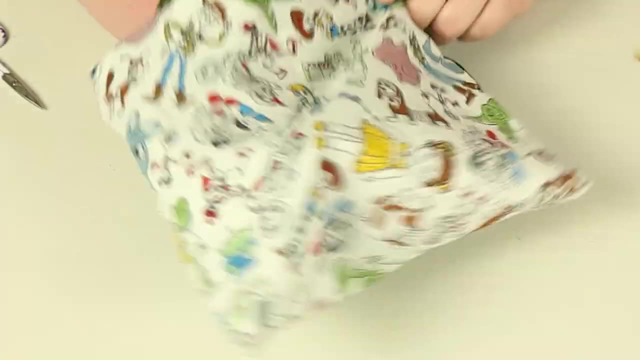 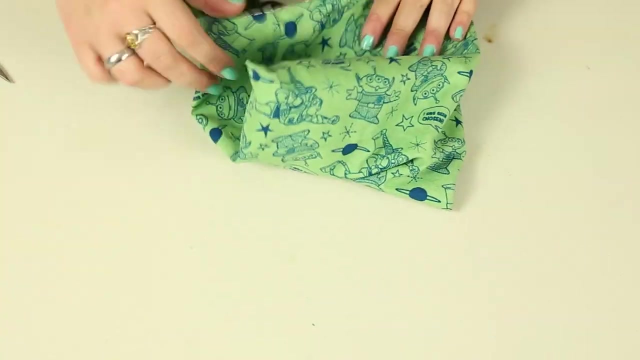 top stitched over the top of that hole just to seal it up, and this is where we simply push the side of the material that's supposed to be the lining into the other side, which is the outside of the bag. now just flip the whole thing inside out so that the lining is on top and bring the corners together. the 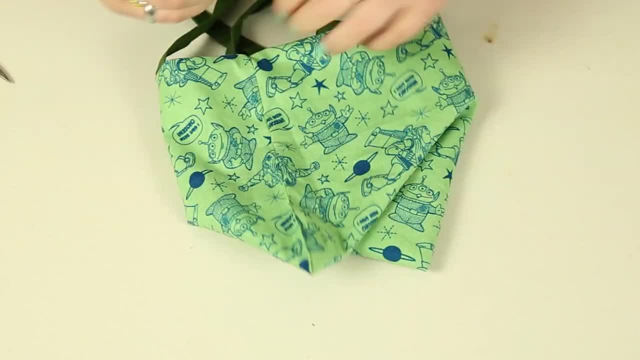 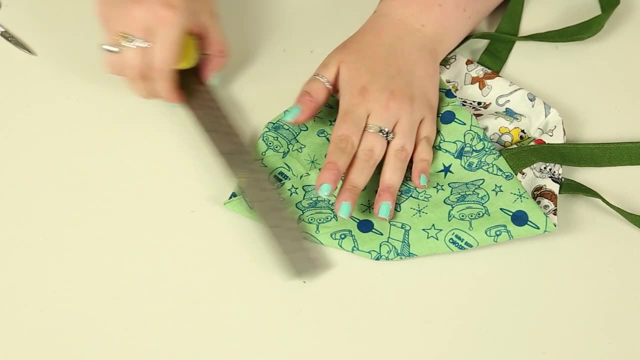 opposite way to which they naturally fall, as you can see here, and draw a line diagonally across about one inch from the bottom on either side, and then just go ahead and sew across that line. to finish off, just to add a little bit more of a professional touch, just top stitch.